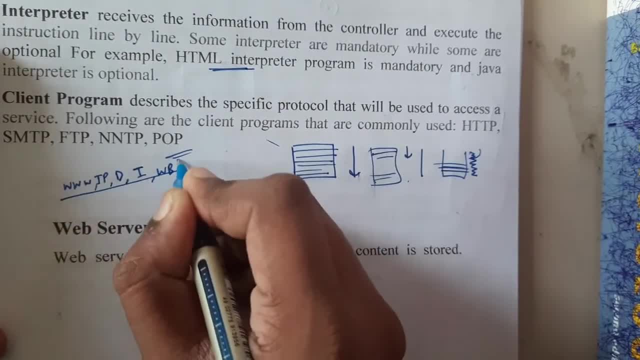 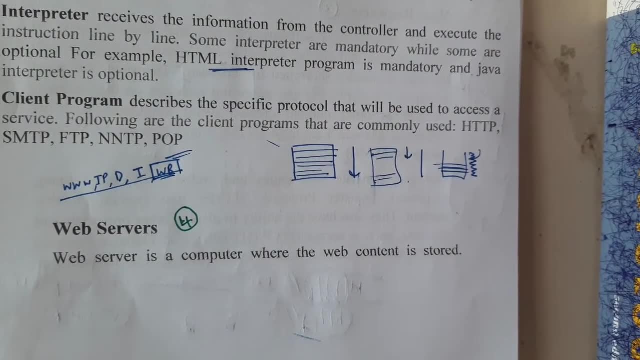 Okay, so these are the topics which we have covered till now. So once we learnt about web browser. so now, what is web server? So whenever someone you ask any kind of web developer, he will be saying that web servers server. there is Apache, Tomcat server. he will be saying that many, many words, right. 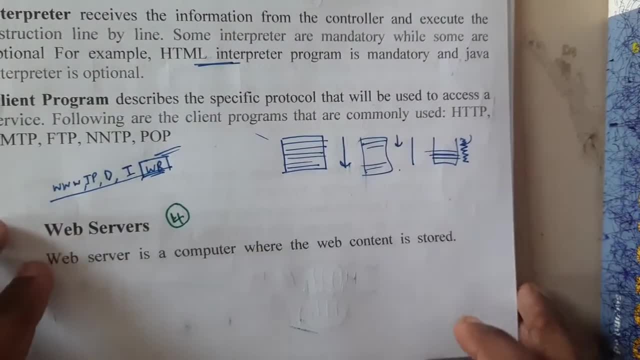 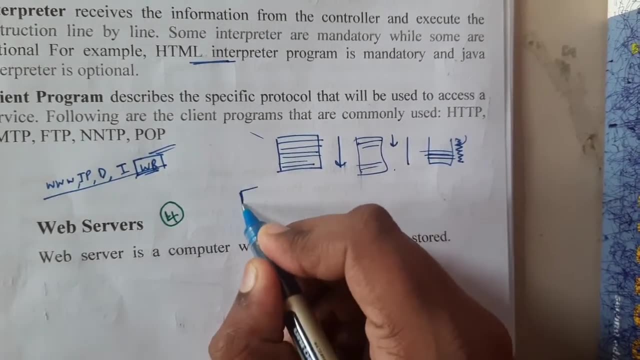 So which will be really unknown for a common user or a common student, right, Okay? so, basically, let us first see what is a web server, So you can assume that it is a computer. guys, it is just a computer, okay. Okay. so let us first see what is a web server. 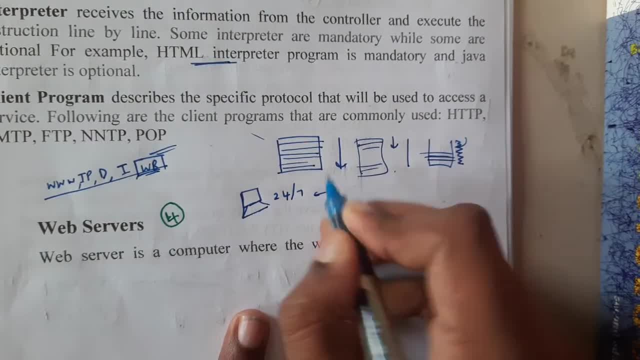 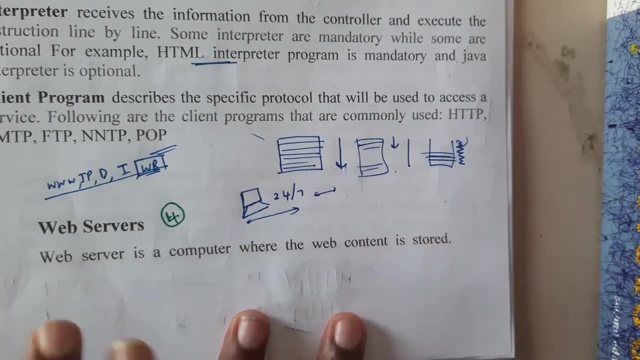 So it will be on 24 by 7,, like every day it will be on. it will never be turned off like a common user. So if you are running a computer, it will be turning off at the night, right So? but these computers will not be turned off at the night. if they are 24 by 7, they will be running continuously. 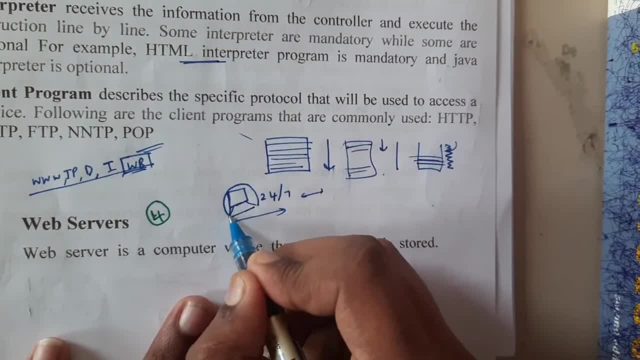 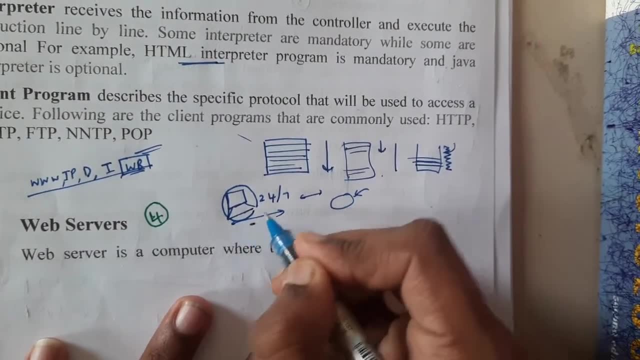 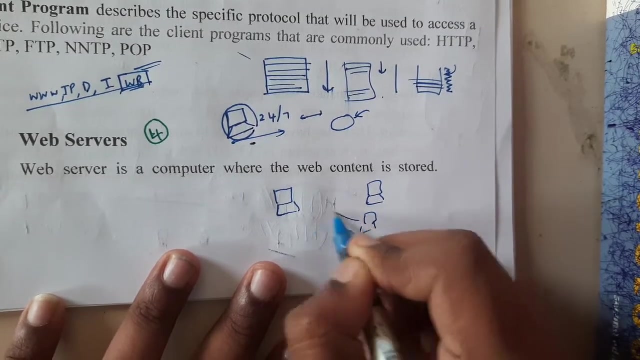 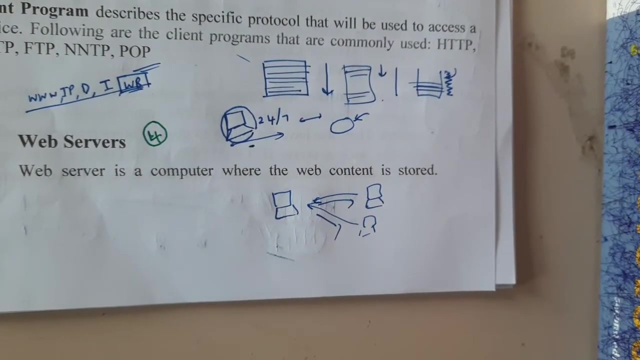 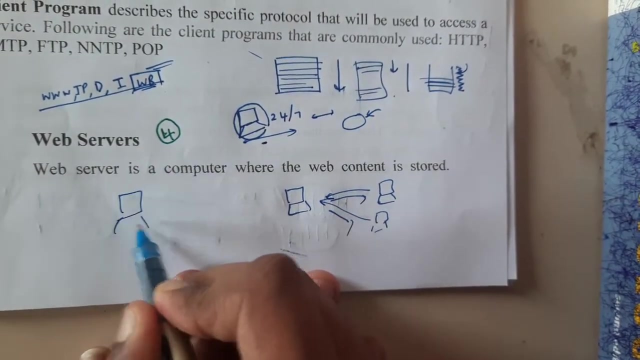 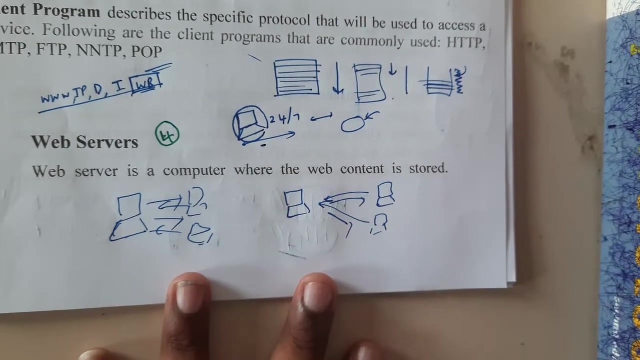 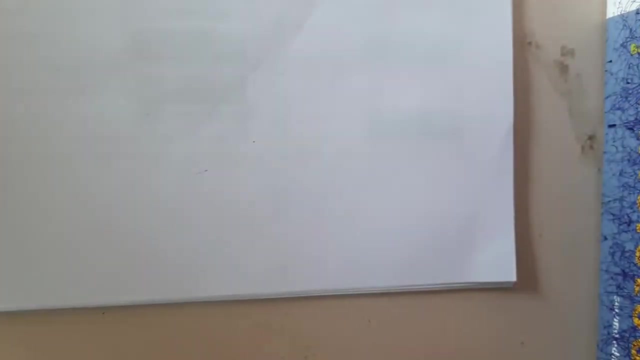 And the main thing is that these systems, or the servers, contains the web pages of the websites. So website web pages are stored here and this system acts as a server. and other people- those are nothing but the users. So web servers will connect to that system to get the data, to collect the data into their system to showcase their website, to show, to open their website. Okay so, once you are going to the theory, you will be getting a clear idea, guys, don't worry. So you can assume that this server will act as a server system which delivers storage or files to the client systems, So there could be a communication between them. Okay so, web server is a computer where the web content is stored. So at that place you will be storing your web content. 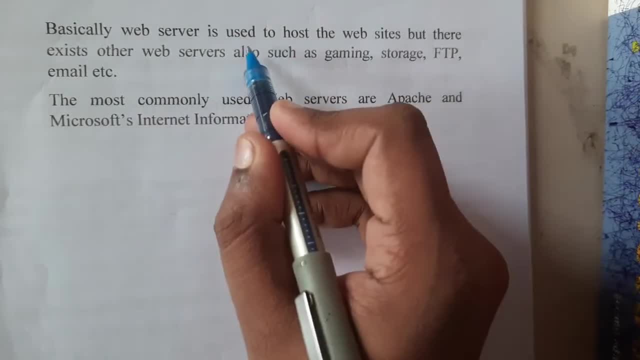 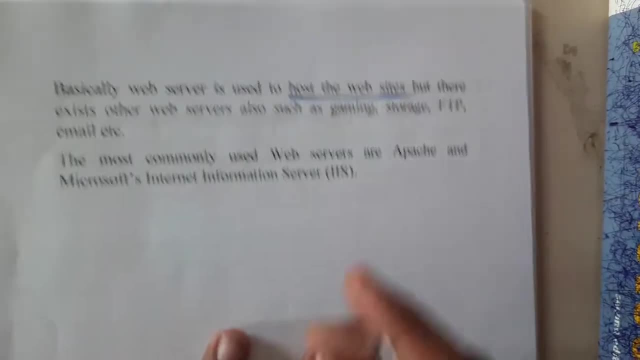 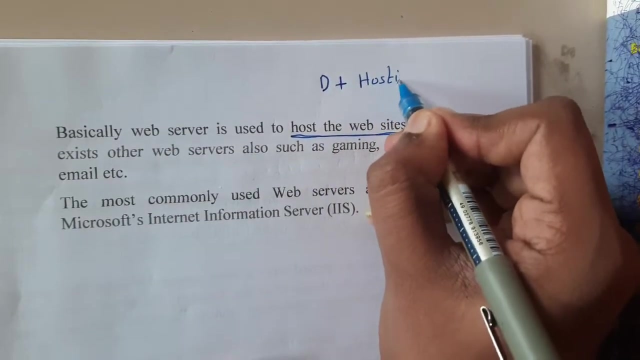 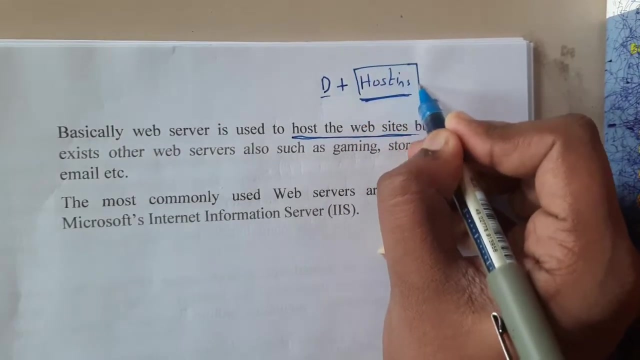 Okay, so basically, web server is used to host a website. Okay, so, basically, whenever you hear someone made a website, so he will be talking about only two things. He will be saying domain name and he will be saying host, hosting a cost. He will be saying the. if you ask him what was the purchases that he made, he will be saying the domain name and he will be saying hosting. So hosting is nothing but the server space guys. So he will be buying some space in some random computer somewhere in the world. 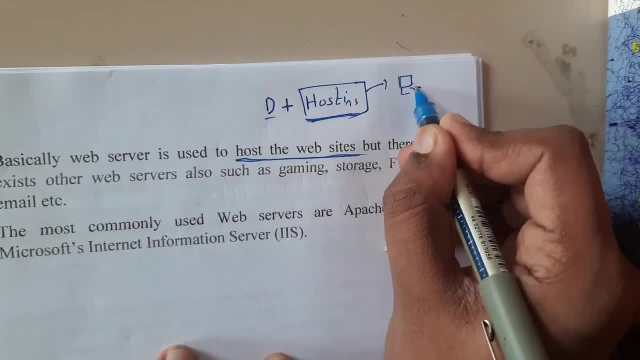 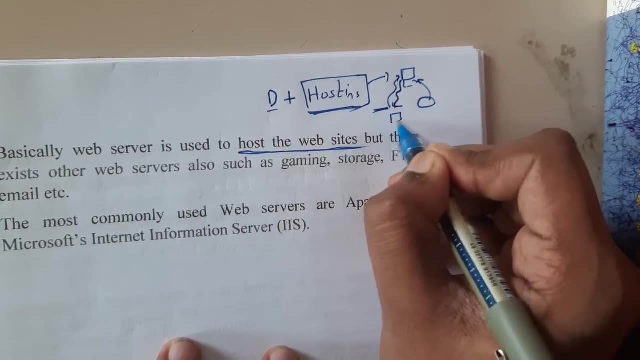 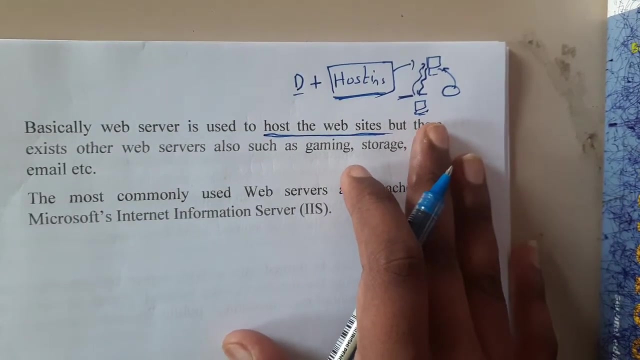 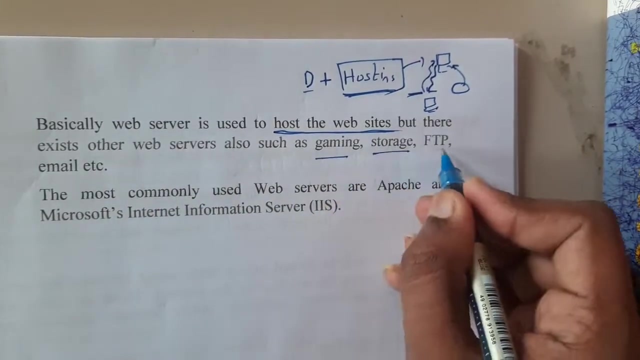 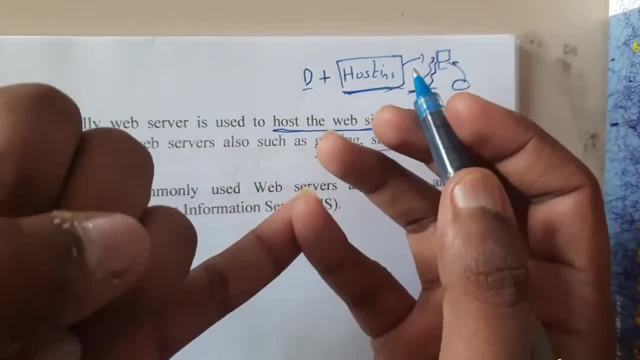 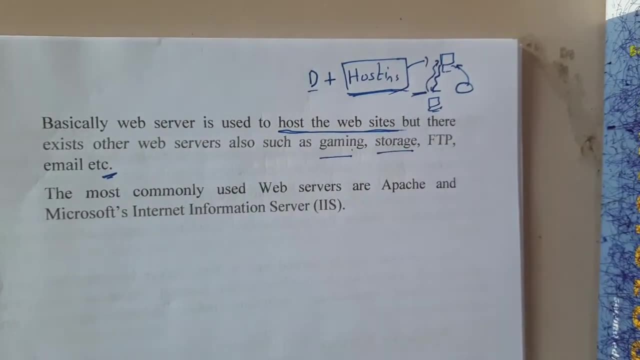 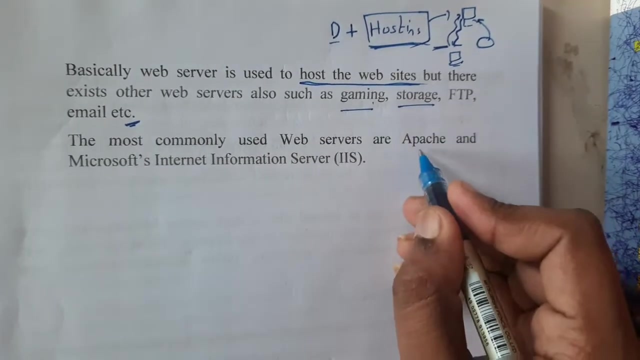 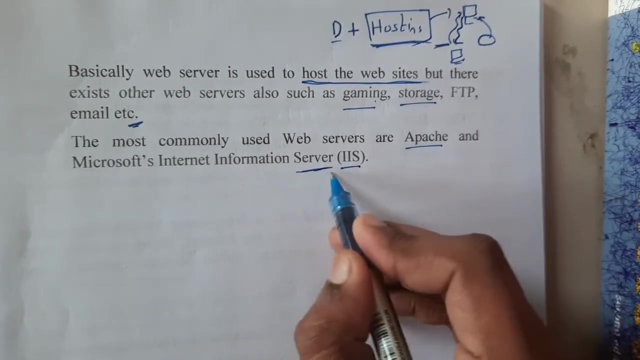 Also run on these kind of servers. You pay PUBG and there are multiple games which are really popular. Okay, so all those games will be having their own servers. on servers, They will be running this and we will be playing like just a user. We are just a client and that is the server. Okay, so the most common web servers are Apache and IIS. That is nothing but Microsoft Internet Information Server. So we'll be discussing about these two like we'll be going through two or three points, guys. Okay, so now. 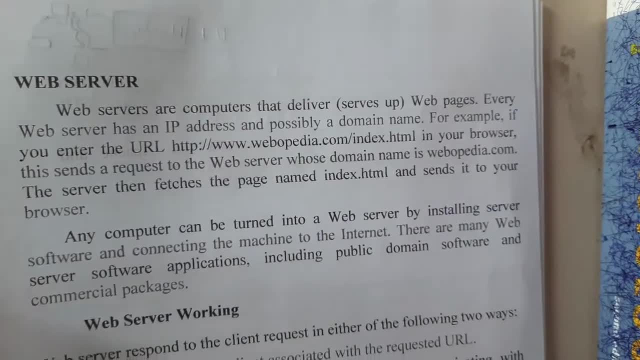 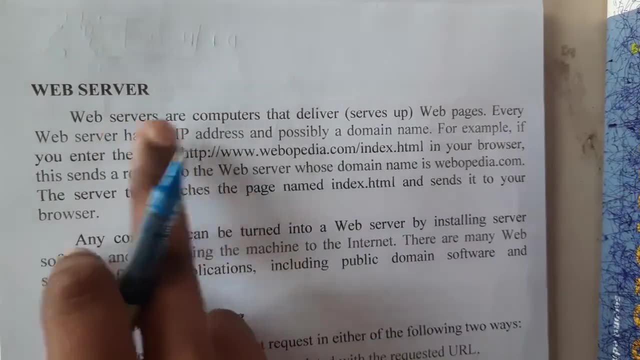 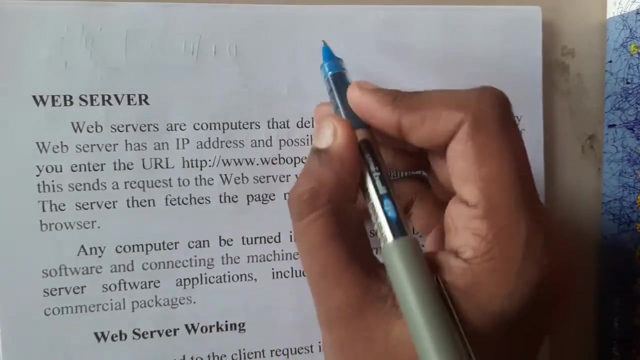 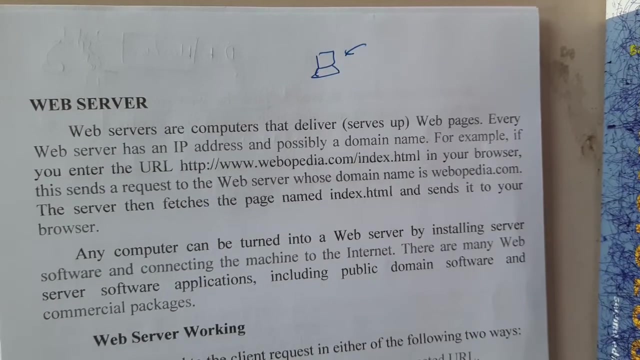 let us go through what is a web server, So we'll be going through some more definitions and we'll be seeing how it will be working internally. Okay, so basically, web server- Web servers are computers that deliver or serves up web pages. So basically I told you so. web server is just a computer in which you will be storing your own websites files. Those are nothing but the HTML files and all those files, and it will be 24 by 7 on. So even if you want, you can make your own. 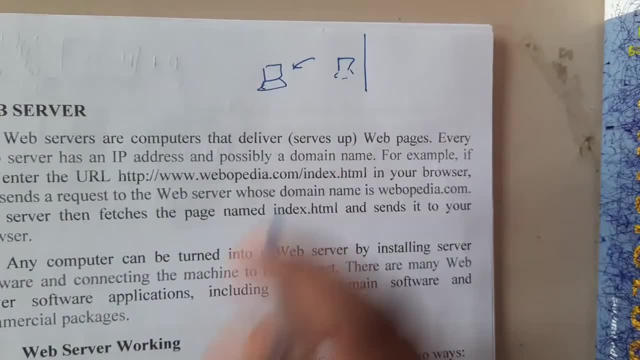 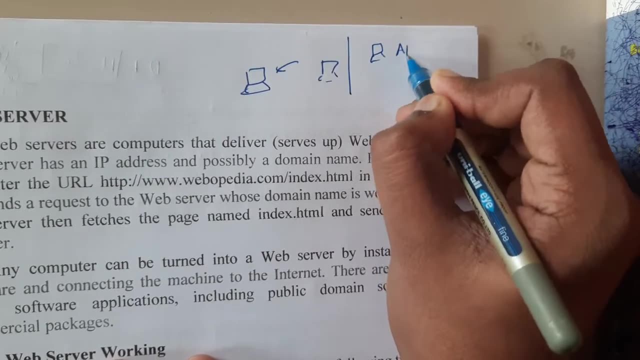 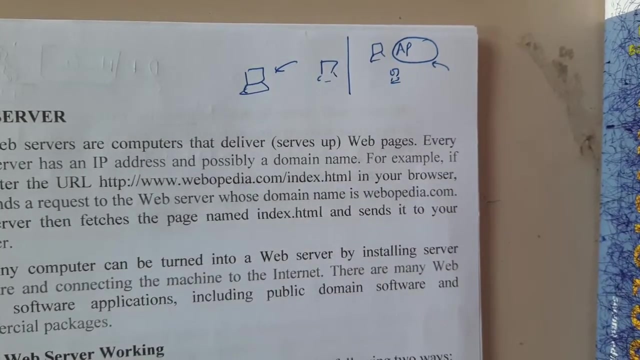 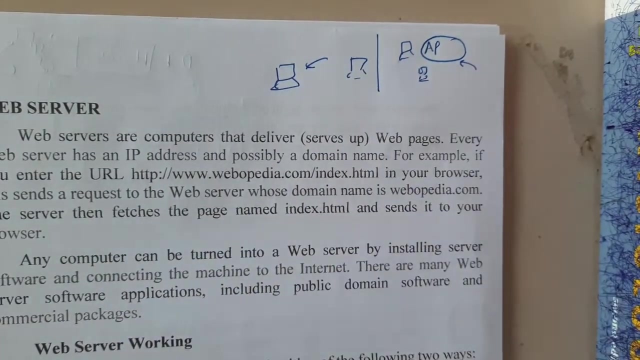 computer as a server guys. So basically, whenever you talk to a developer, like if you talk to a web developer, he will be saying that my system, in my system, I am having Apache Tomcat- he'll be saying that that is a local server, guys. So your system will act as a server and you can run the whole application on your system only, without buying any kind of hosting space or any space. So basically, in the initial stages they will be using this method to start their development. Okay so web servers are computers that deliver or serves up web pages. 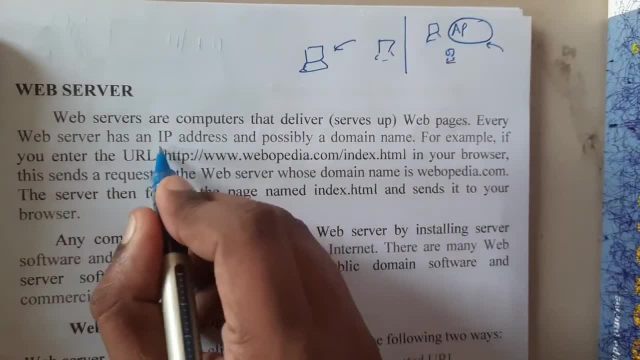 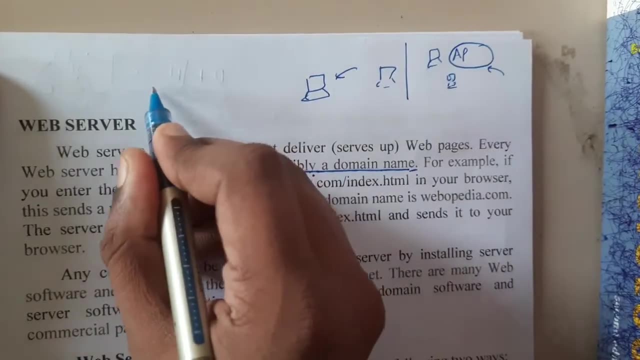 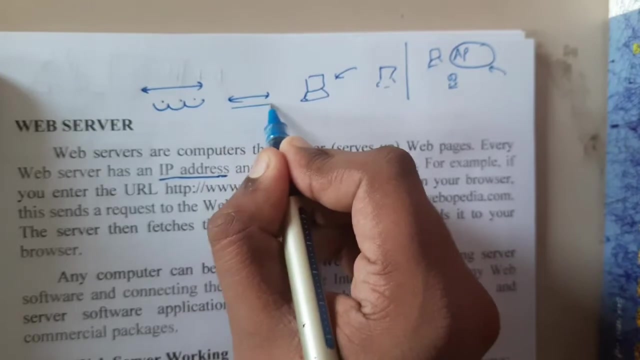 so every web server has a particular ip address and a possible domain name. so basically, we discussed about ip address and domain name. so ip address is nothing but numbers which are of four pair, four pair, and we are having the domain name. that is nothing but wwwsomethingcom. okay. 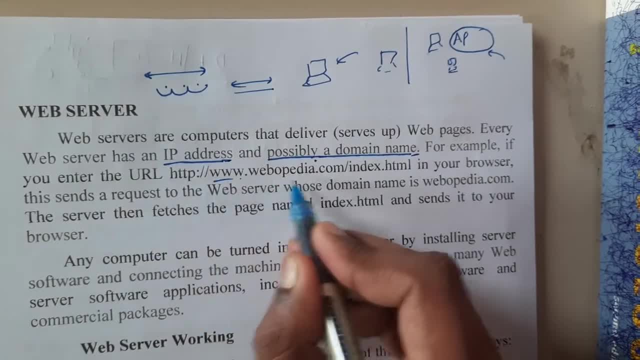 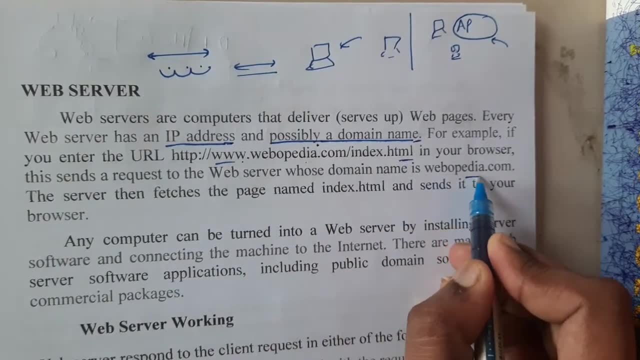 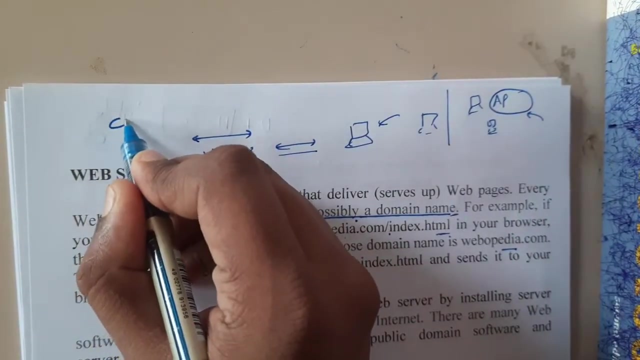 so, for example, if you enter a url, so assume this is a url you have entered in your web browser. this sends the request to the web browser whose domain name is that. for that it will be sending the request, and please remember that, guys, please remember this whenever you open a website. the 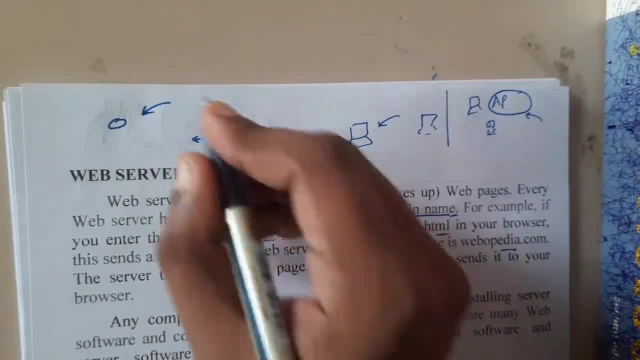 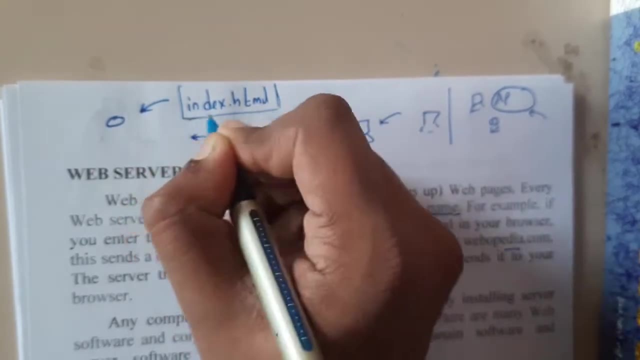 first file, the first html file- that is nothing but home page file- will be in the form indexhtml guys. so basically, this is the format which we will be using. like, this is the file name which you should use for the home page. like, basically, when someone visits your website without anything. 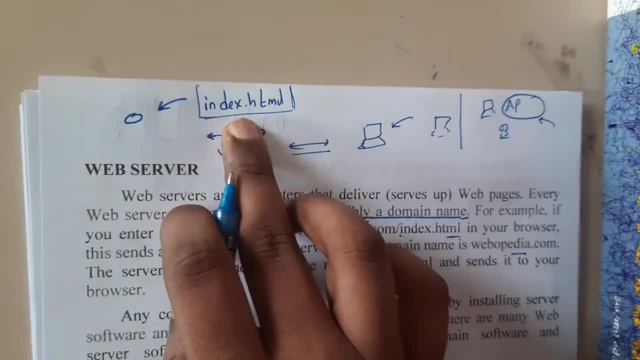 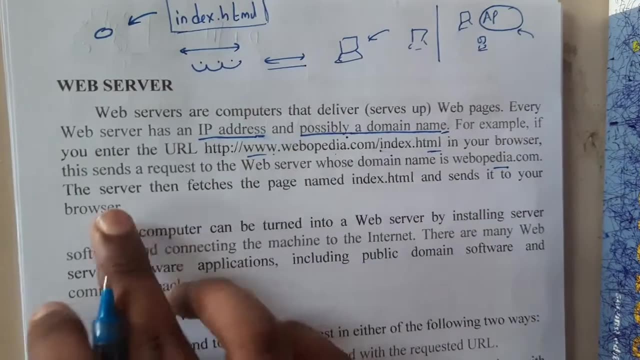 continuous like slash. that's it. he will be directly redirected to indexhtml. so that is the use of indexhtml. we'll be discussing about that in, i think, third or fourth unit guys, don't worry okay. so the server fetches the pages named indexhtml and send it to the browser. so basically, i told you right. 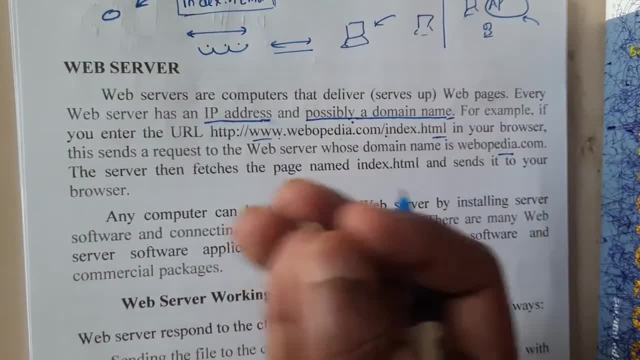 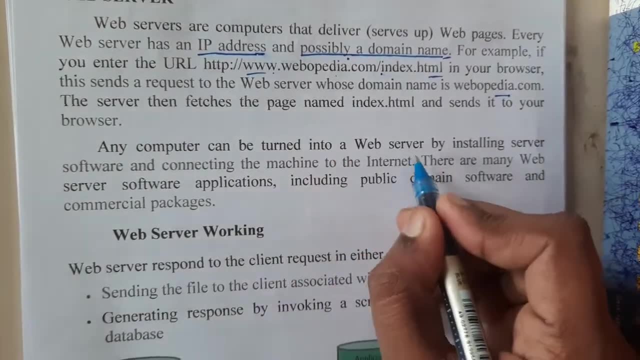 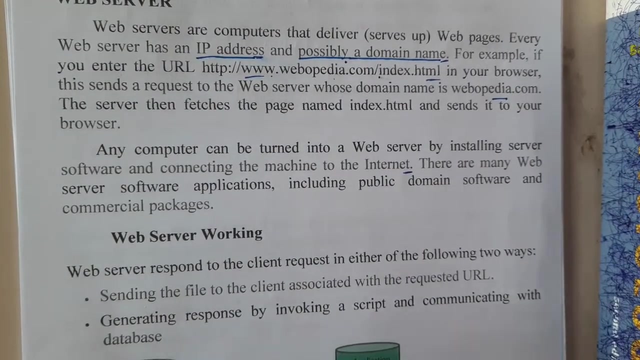 it will be downloading or it will be collecting there from and it will be sending to the user. okay, sorry for that. any computer can turn into a web server by installing the software and connectivity machines, connectivity and connecting the machine through the internet. so basically, i told you right by using apache, tomcat. 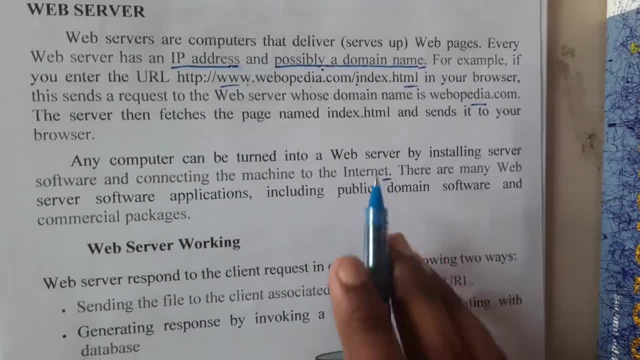 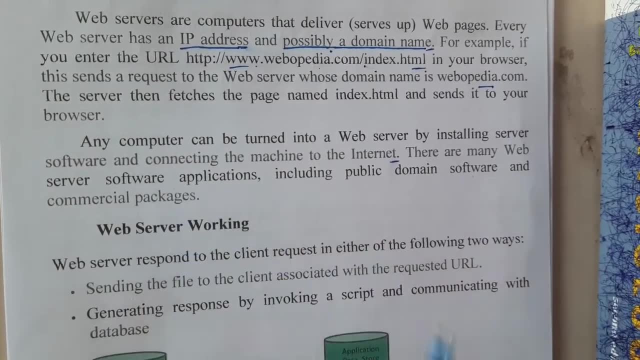 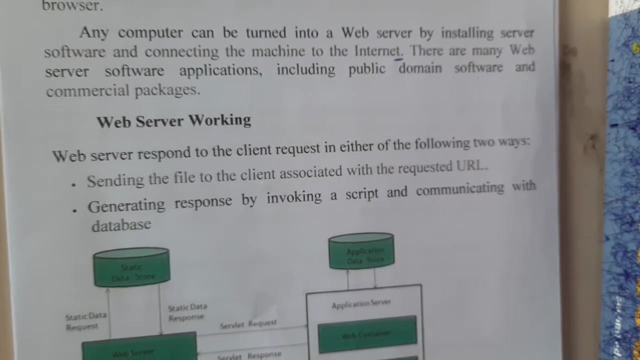 that is the popular server for web guys. okay, so web servers by initializing the software. okay, there are many server software applications, including public domain softwares and commercial packages. okay, so web server working. so how the web server will work. so basically, you will be thinking that, okay, it will be a median in between both right to the storage and to the client. yes, you are correct. 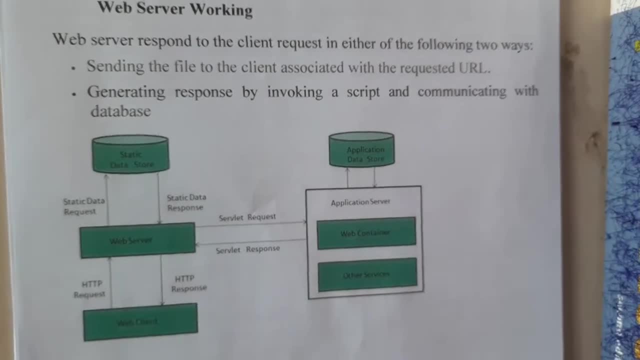 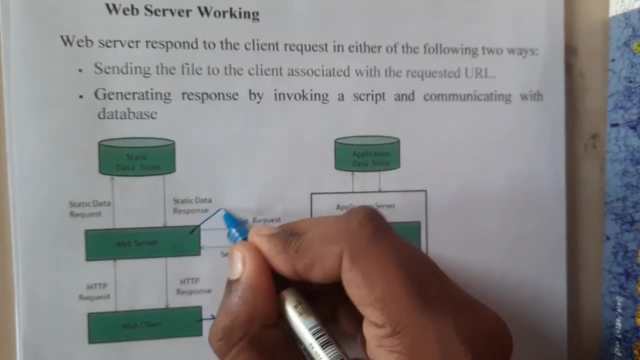 but there is some more twist in it, so okay. so now let's see how the web server will work. so, basically, i think the image is not very clear. i'll be, i'll be just saying you the words: guys, so this is nothing but a web client. guys, this is nothing but a web server. this is nothing but static data storage. 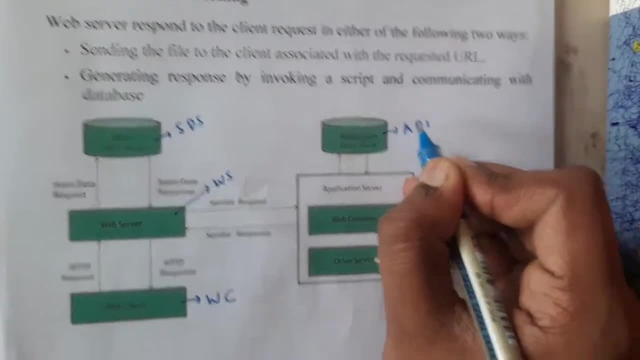 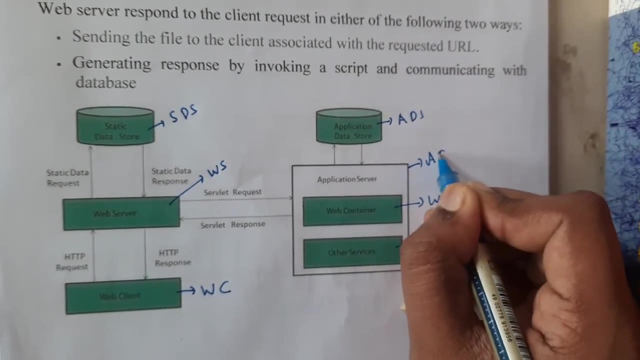 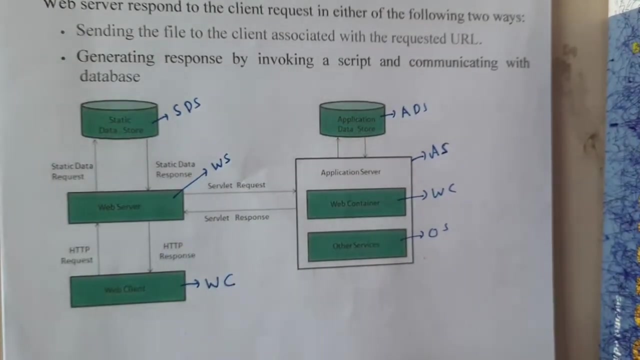 this is nothing but application data storage. this is web content. this is other services. this is application server. okay, so basically, i have just written in the shortcuts: guys, please stop pause the video whenever you want and you note it down and you will. you draw the diagram, okay. 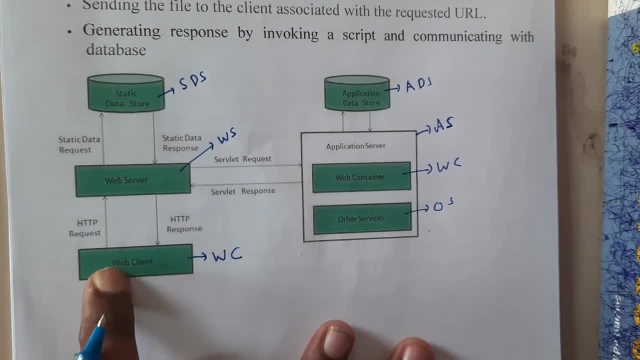 so basically, here we will be the client, we are the users. so we will be initially requesting for a website. so assume that i wrote wwwgooglecom, so the request goes to the server. so basically there is an intermediate process. guys, if you want, i will be, i'll be teaching you that also. so once you type, 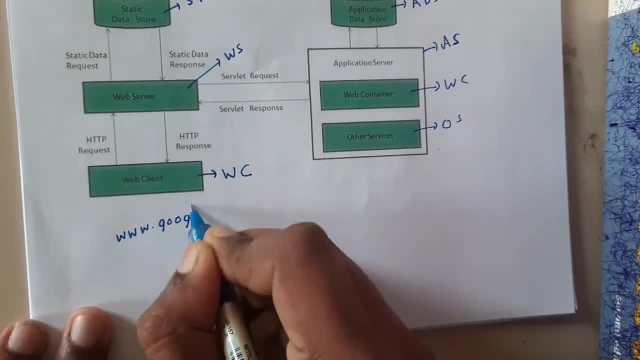 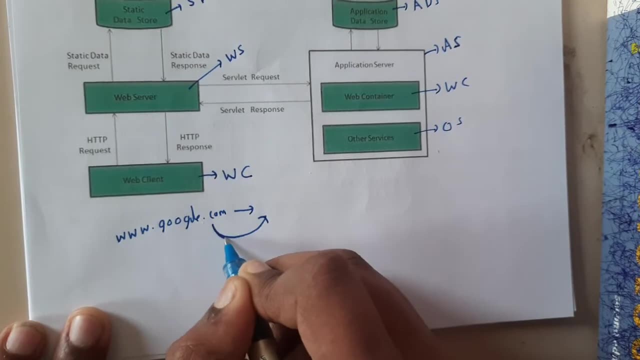 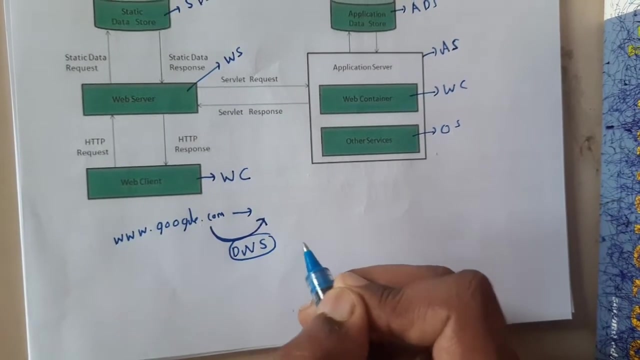 wwwgooglecom. okay, so initially it checks the ip address of this, so it converts the name domain name into ip address. so this process is the process of converting the domain name into the ip address. so this process is the process of converting the domain name into the ip address. so basically, 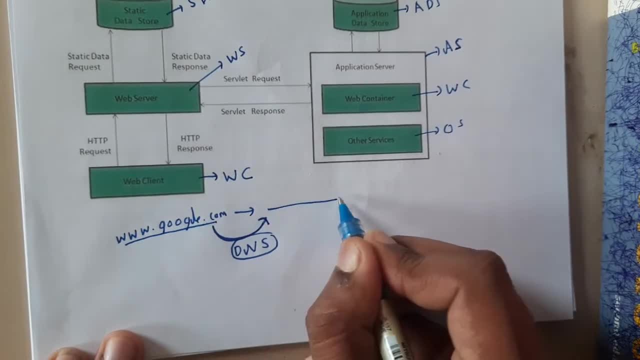 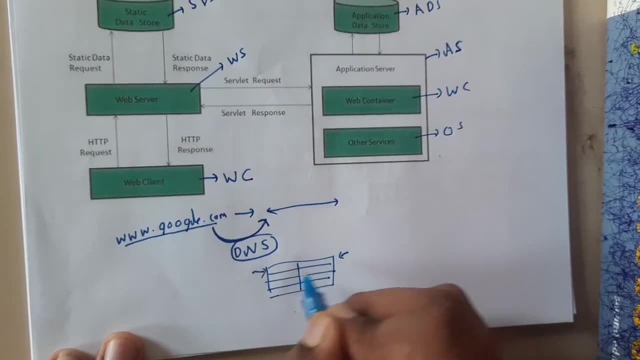 each and every domain name will be having a corresponding ip address. so all these ip addresses are stored in a table. you can assume in that way for now, basically like a telephone directory. you will be having the name, phone number, similarly the domain name and the ip address. so this records is. 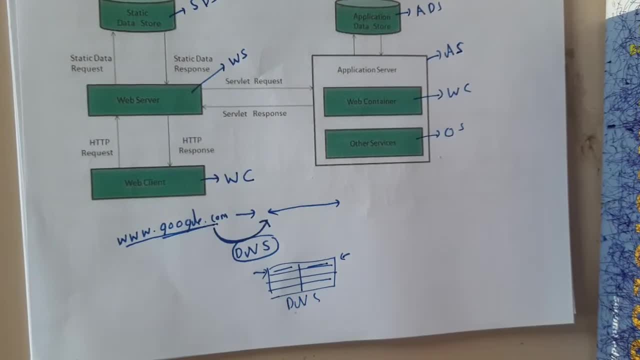 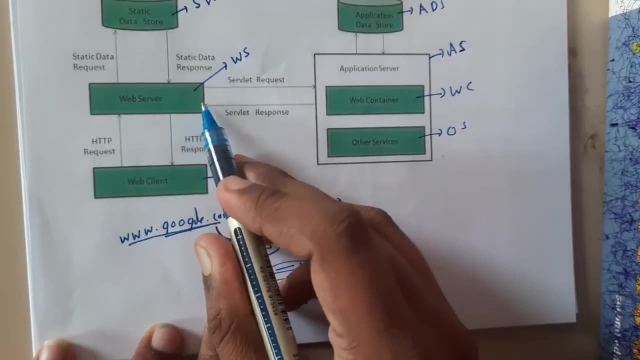 called as domain name records or domain name server. they will be saying some people will be saying domain name system, server service. also they will be saying, okay, so from the ip address now you will be going to the server. so you requested, finally to the server. so, based on your request, 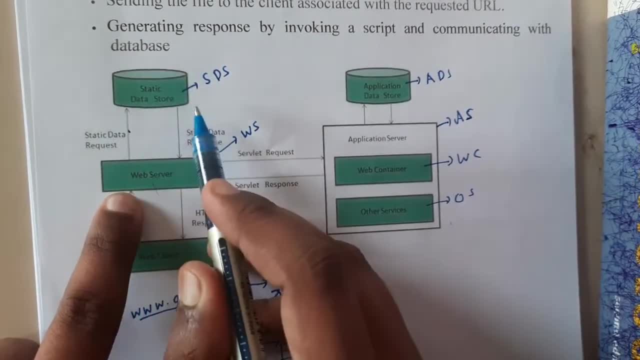 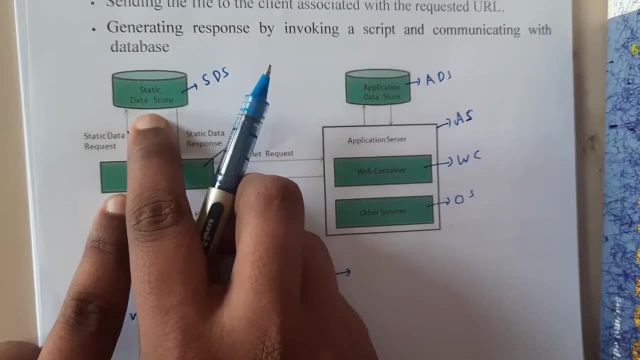 if there is any static data like that, this, this static data, you can assume it as a constant data. there will be no updating in it, okay? so if you request for that data, it will automatically collecting from there and it will be giving you the response and you'll be getting the response. 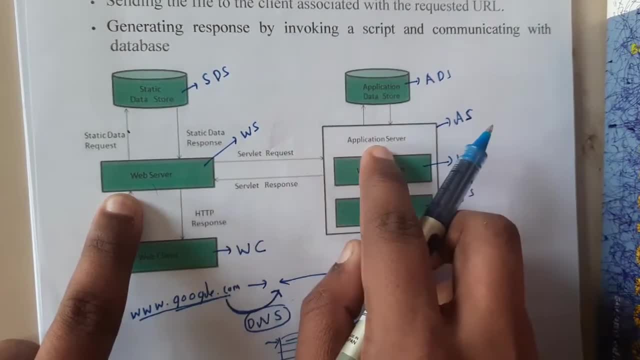 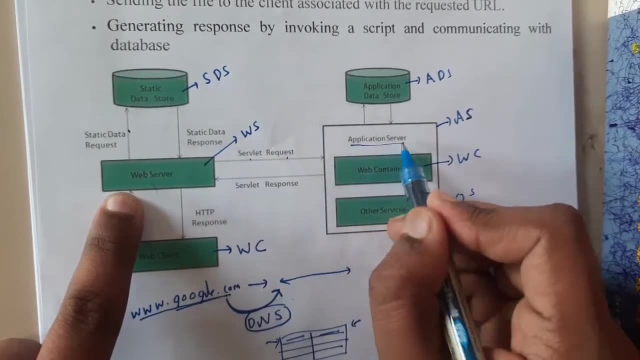 if not, you are directly trying to do something with the application, like you're uploading a file that should go into database storage, right? so that is the reason why it will be going in this path. that is nothing but server request. you'll be going to the application server. you'll be checking the. 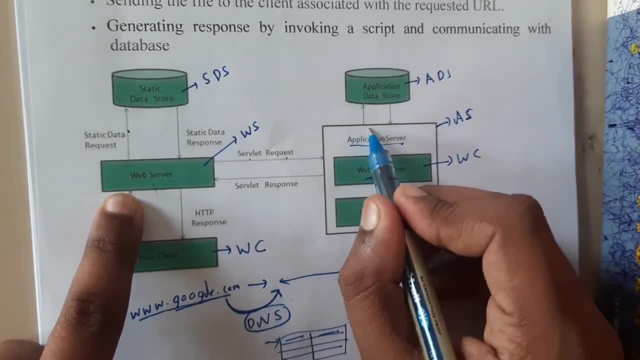 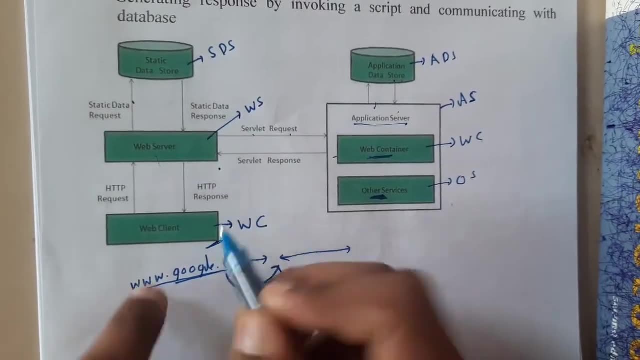 web content and any other services and if you do any modifications, that will be reflected in the application data storage. okay, and you'll be getting the response back and you'll be, finally you'll be receiving the website on your face, on your, on your face of the computer, okay, so i hope. 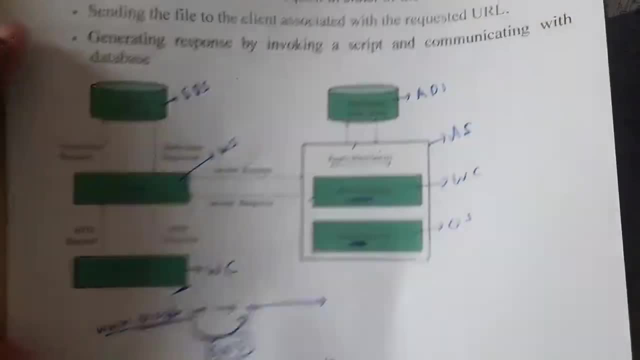 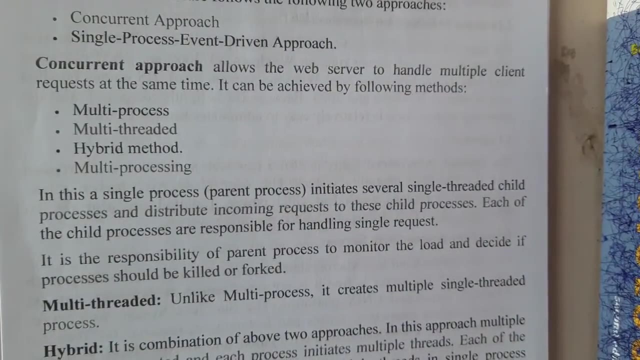 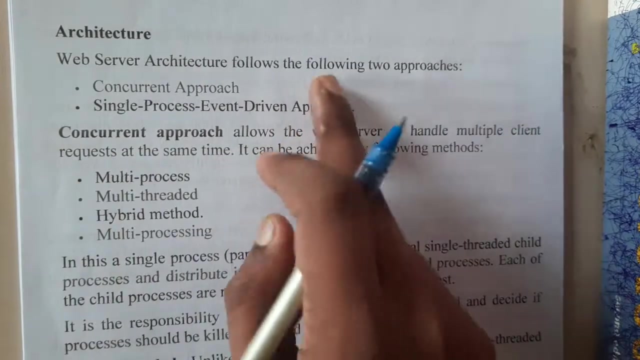 everyone got a small idea on the working of the web server. okay, so now let us see the overview of architecture. guys, because i also didn't find the exact theory for this architecture, so i have just copied it from a file. okay, so architecture. so web architecture follows the following two approaches. there are two main. 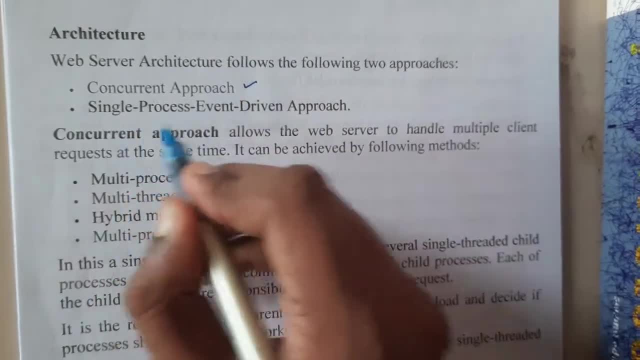 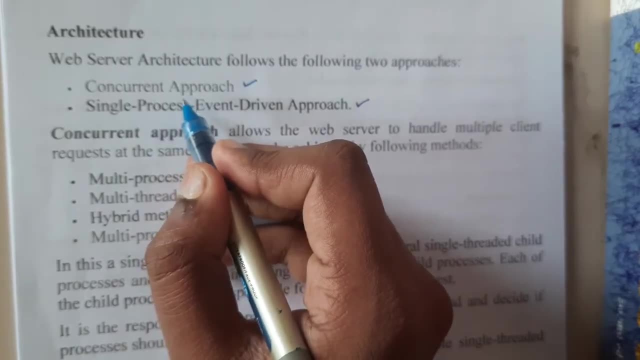 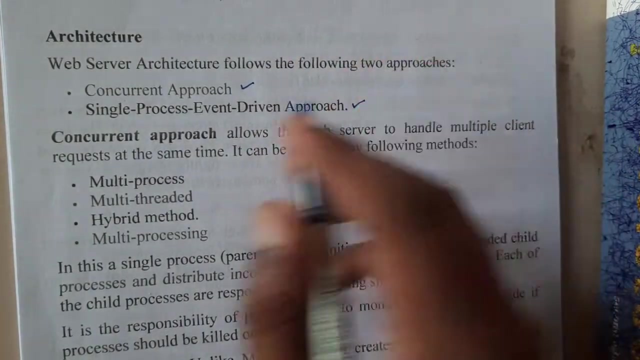 approaches guys. that is nothing but concurrent approach and single process- event driven approach. so basically from the name itself you can say: concurrent approach means you are trying to concurrently give access to multiple things, like using threads or multi-threading or some concepts like that, and single processed even means you are giving only one guy, so only one guy will come in. 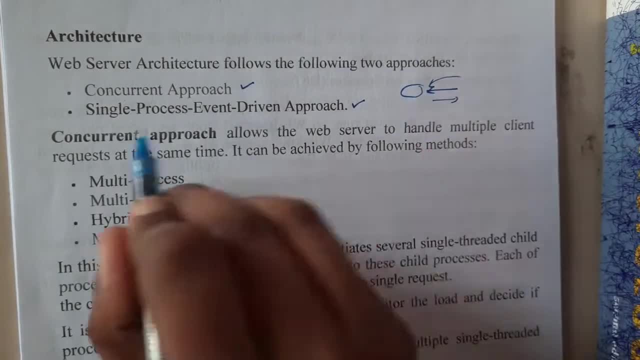 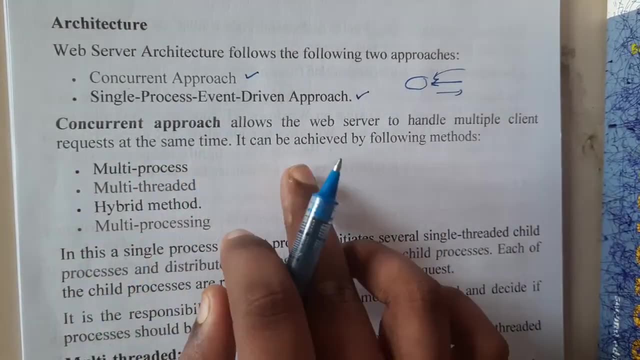 he'll be collecting his data going back again. then only new guy will come, like that single process. okay. so concurrent approach allows the web server to handle multiple client requests at the same time. it can be achieved by the methods of threads. so basically, assume a big server guys. 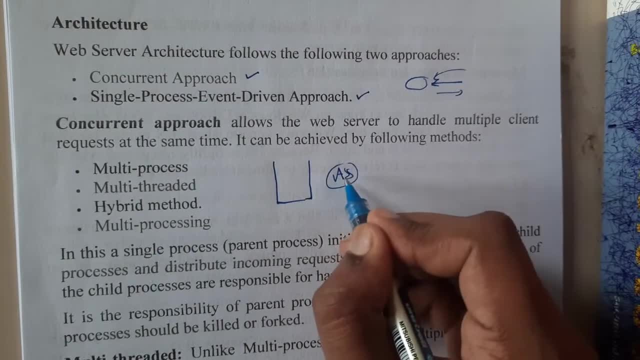 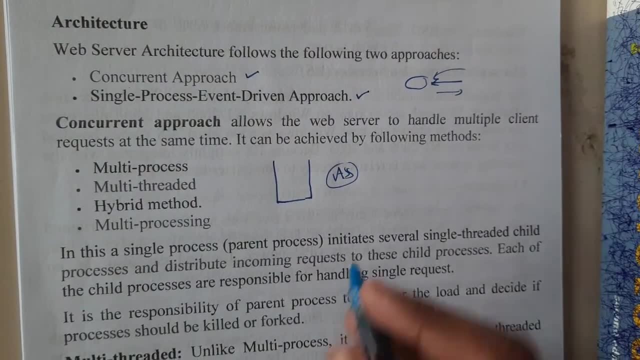 like you are the owner of amazon company. okay, so your amazon? will there be only a single user at a time? guys, there will be some thousands or lakhs of users at a time on the website, so each and every one's request should be accepted, right, so there should not be no discrimination. that. 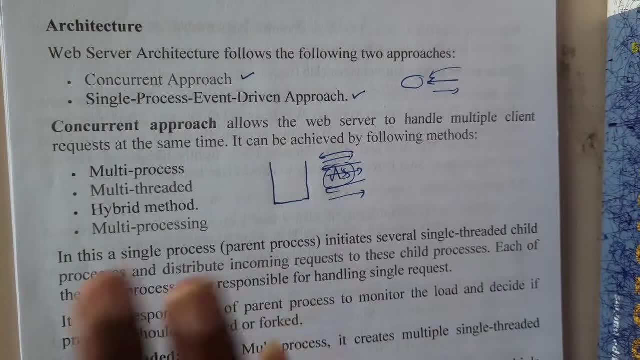 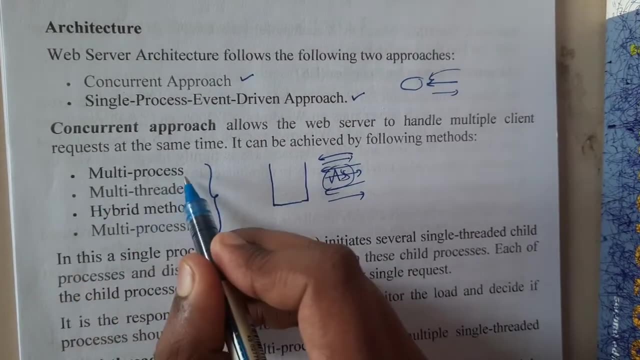 you are not allowed. you are allowed. You will be given high priority like that. No, Everyone will be given the equal priority. by using these concepts will be used guys. He will be using multi process or multi thread or hybrid methods or any kind of multi processing methods. 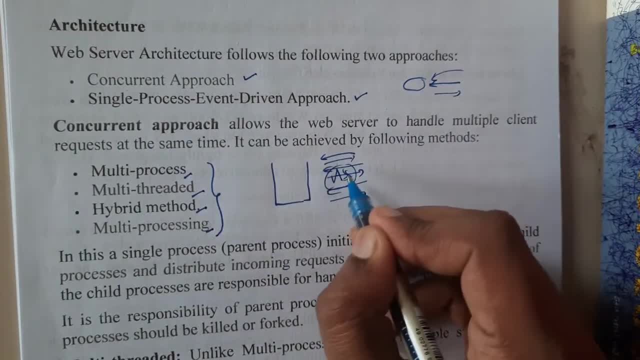 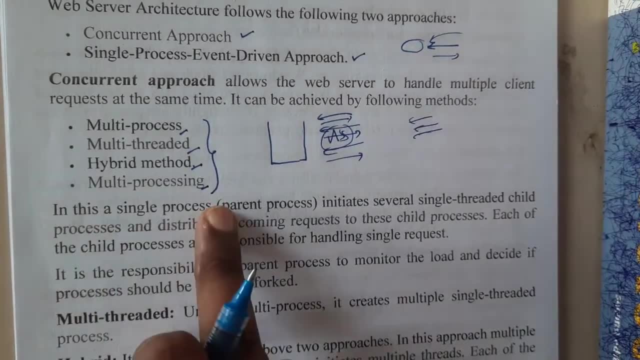 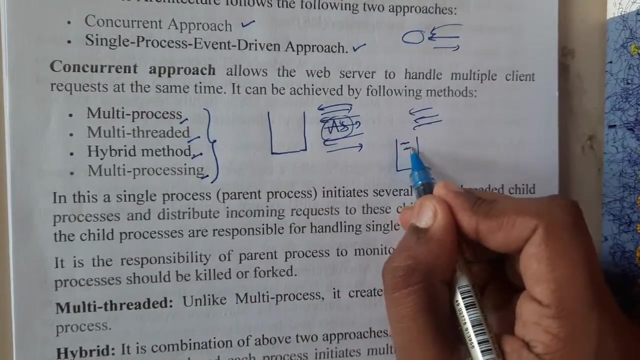 So these are the different methods he can use to make this achievement. like multiple users can access at the same time and request for the for anything as per the requirement. Okay, So in a single process, parent process initiates several single threads. So basically the parent process will create several threads. like assume there are 10 threads. 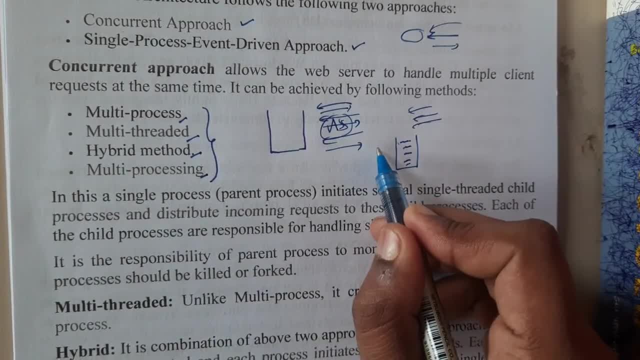 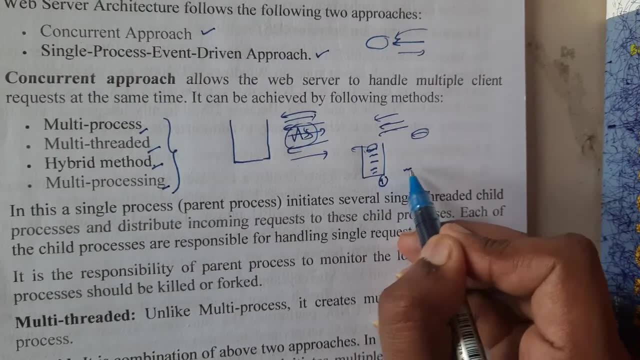 Okay, So each thread can take the particular task. So basically, first user comes, he will be taking the first thread and he'll be going. So now we are left with nine. So in that way, till one once zero. after that the server will be slow. 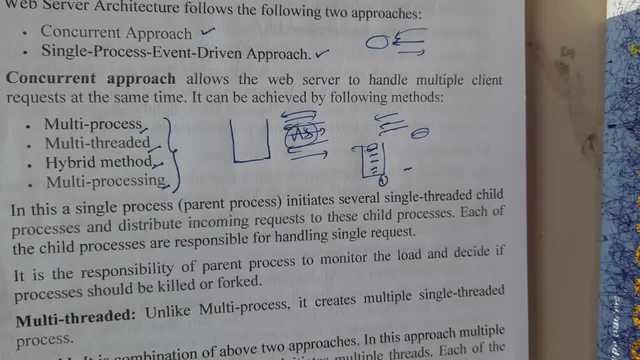 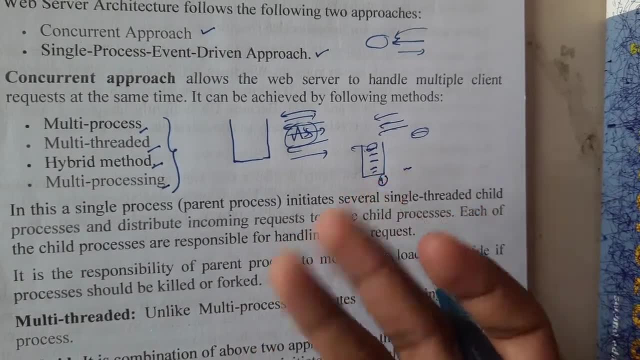 So we will be getting right timeout, 404, network page issue like that. There will be many, many kinds of issues, Right, So those issues you'll be getting, or the server will be, cannot handle that much burden. Okay. So, whereas in reality 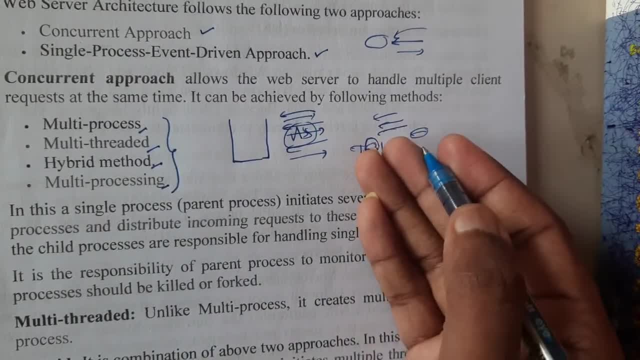 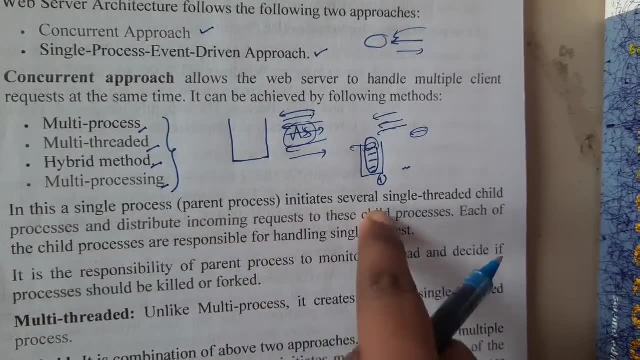 There will be many threads, guys, not even 10. there will be some thousands of threads which can handle each and every request. Okay, So at a time. So in this single process that is nothing but parent process, initiates several single threads, child process and distributes incoming requests to the child, 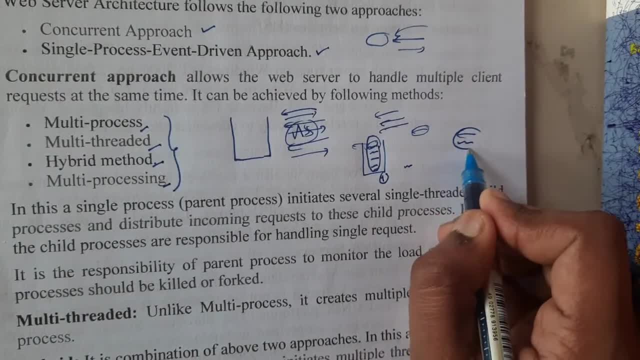 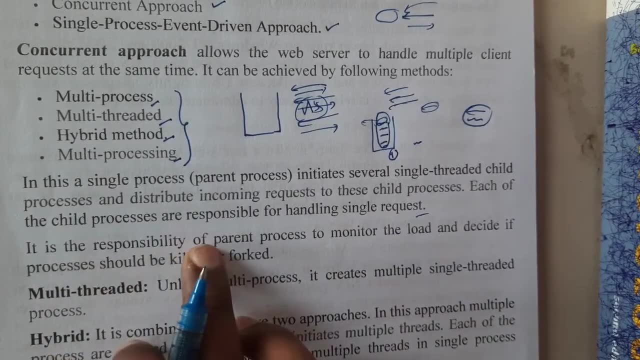 So whenever a request come, a child will be allocated. there is nothing but a thread is allocated for it. Okay, Each of the child process are responsible for handling a single request in this. it is responsibility of a parent process to monitor the load and they decide. 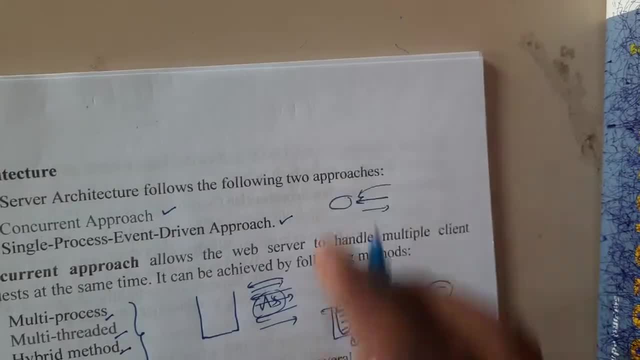 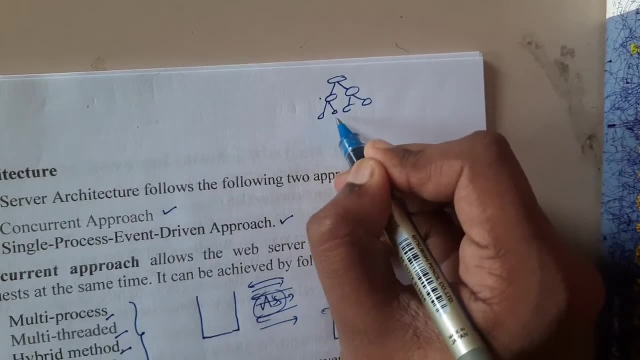 You put: If processes should kill or fork forked, kill is nothing, but you'll be. so assume that you are doing: fork fork is nothing, but you are creating duplicates guys. then you are increasing the number of threads, So assume that you are. you are having a huge server, but the customers or clients you will be getting only one or two per day. 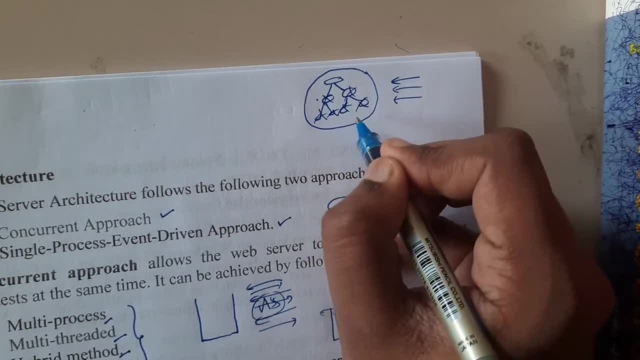 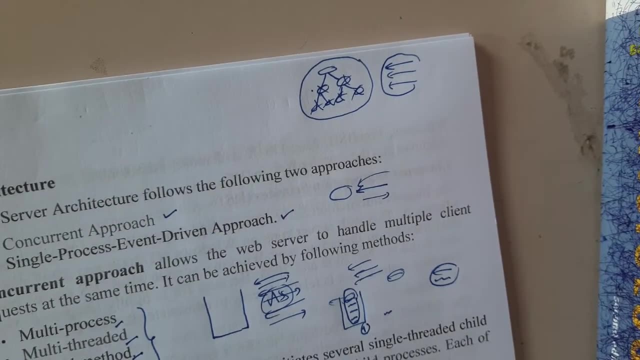 Then what is the need of this much? you need to kill them. So in that situation, you'll be killing. So this killing concept will be applied at night times, guys. basically, at night times, most of the users will not be interacting with most of the websites, so they'll be killing the threads. 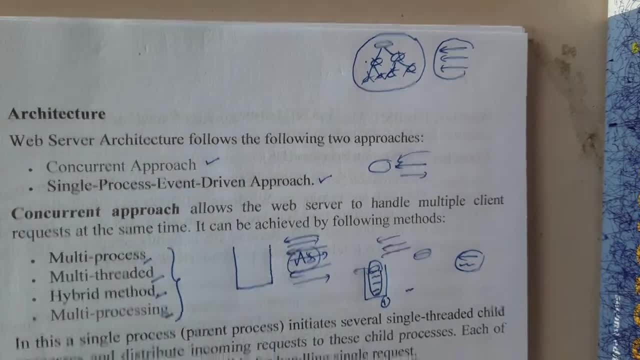 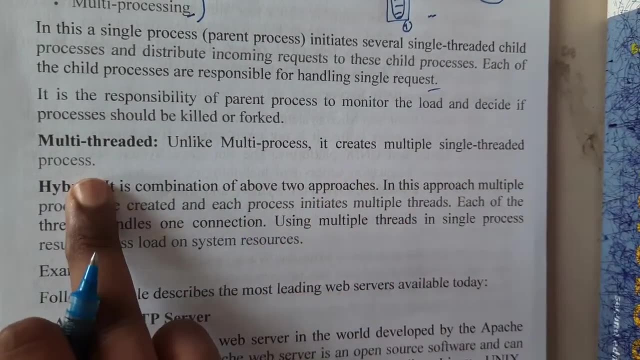 And again at the morning they'll be forking them so that it will be beneficial for them. Okay So, multi threading. unlike multi process, it creates a single threaded process. Okay So, hybrid, it is a combination of both the processing- multi process and multi thread. 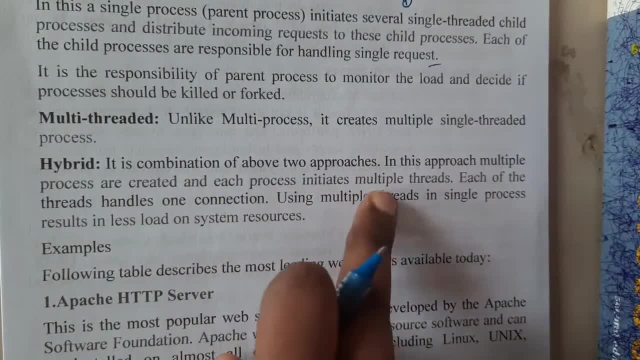 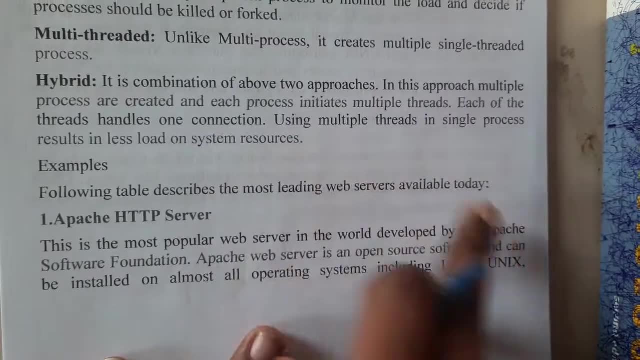 Okay, In this approach, multiple processes are created and each process initiates multiple threads. So this is what I've just told you guys. Okay, So this is what I've just told you, because each process will be taking a particular thread and they'll be solving it, so using multiple threads in a single. 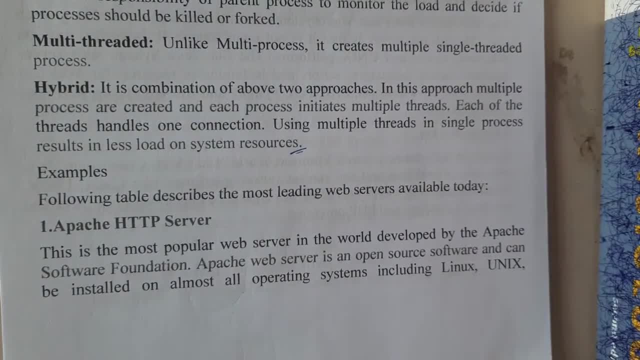 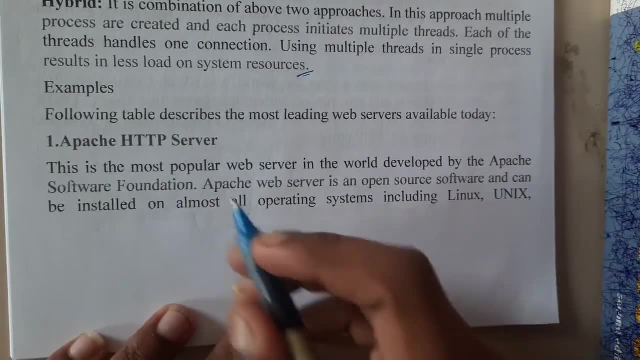 Process. it will send less load on the system. So at the end you will be ending up with the less load on the system. Okay, So we are having multiple popular servers, guys, so we'll be discussing what three to four servers here. So the first is Apache. 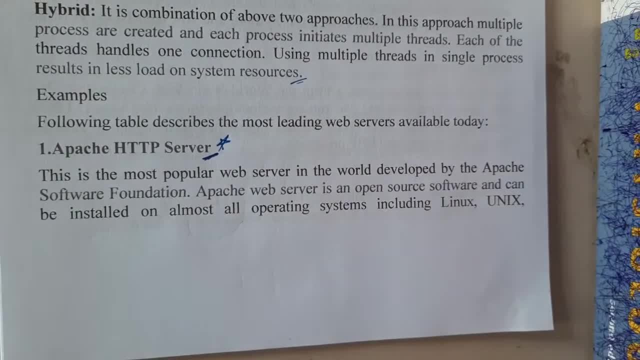 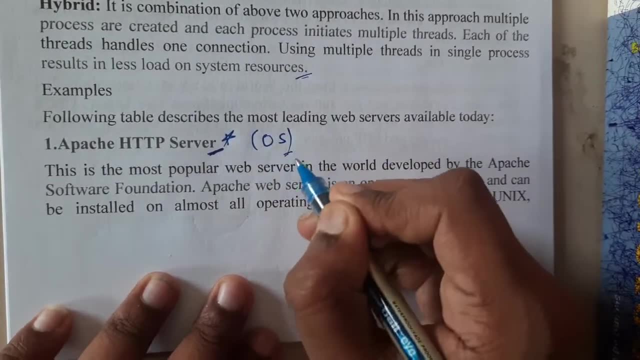 So, if anyone, anyone, you can ask us, because Apache is one of the most powerful and popular. The main reason behind Apache being popular is nothing, but it is open source. Okay, This is open source. you can do any kind of modifications as per your requirements. 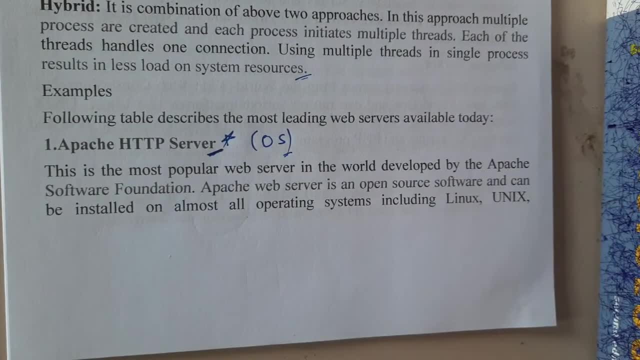 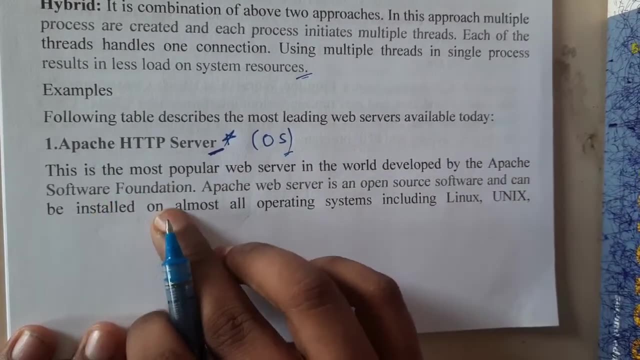 If you don't like a single feature in it, you can change it, If you are good at that much. if you are good at coding, you can do it. Okay. So this is the most popular web server in the world, developed by Apache Software Foundation. 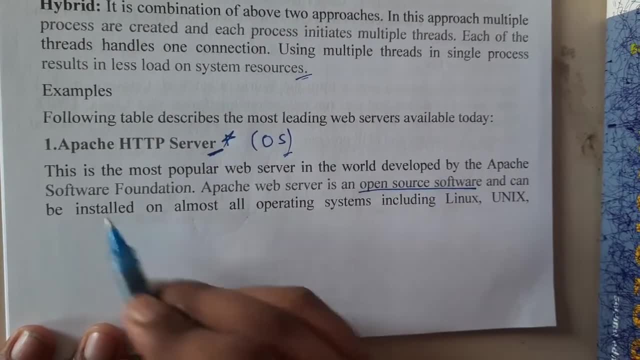 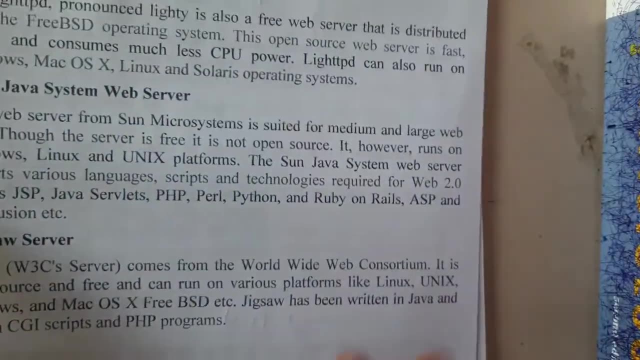 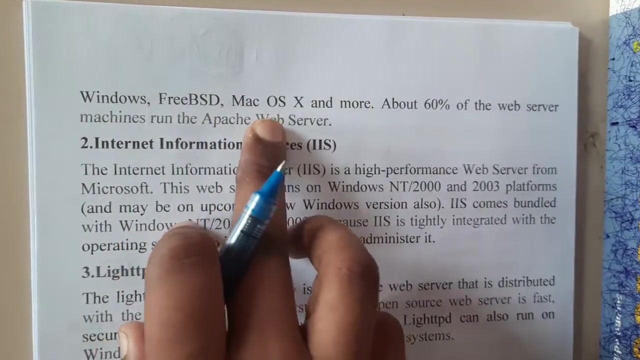 Apache web server is an open source software and can be initialized in almost every operating system, including Linux, Unix, anywhere you can initialize the software, So even for local working also, we will be using Apache Tomcat server. Okay, Okay, So Windows, FreeBSD, Mac OS X and more. 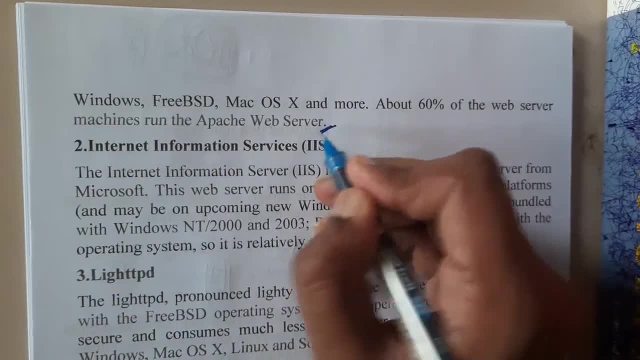 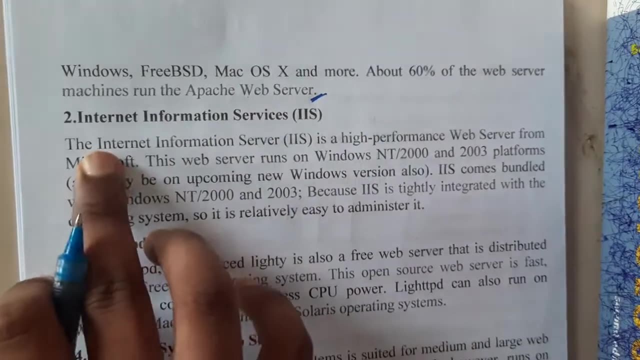 So about 60 percent of the web. Okay, Web server machines run Apache only above 60 percent. Okay, Okay. So Internet Information Service- This is for this is from Microsoft guys. So the IIS is a high performance of web server from Microsoft. 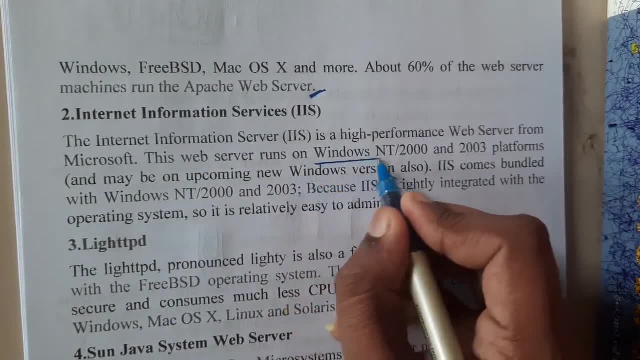 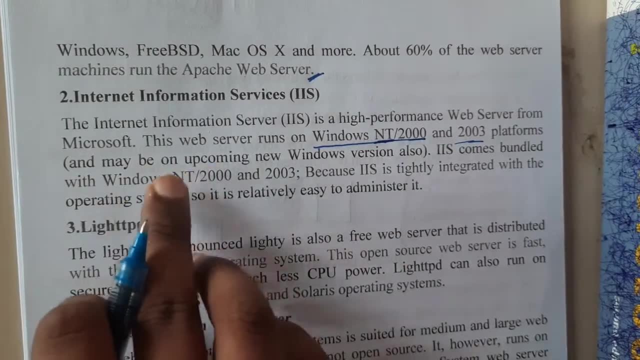 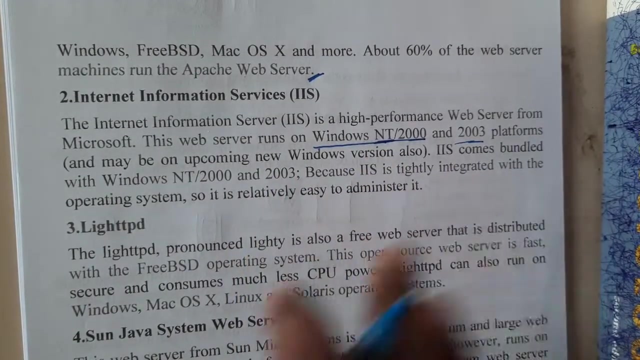 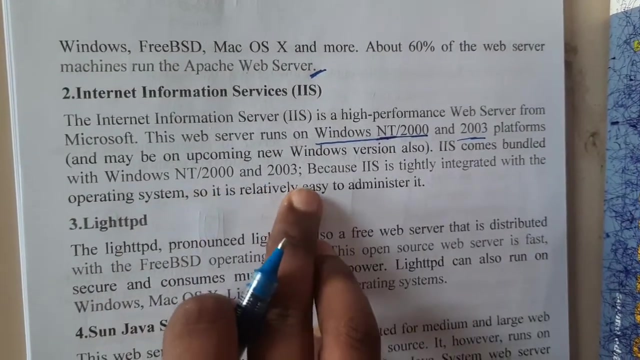 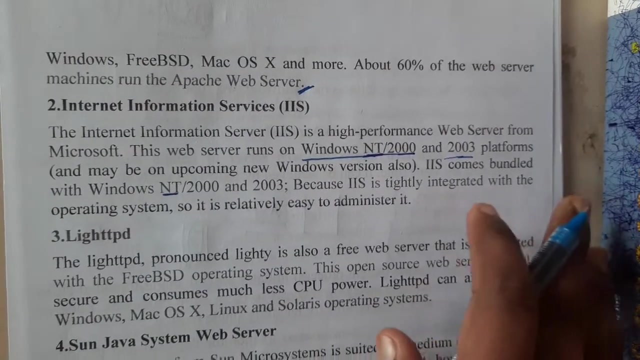 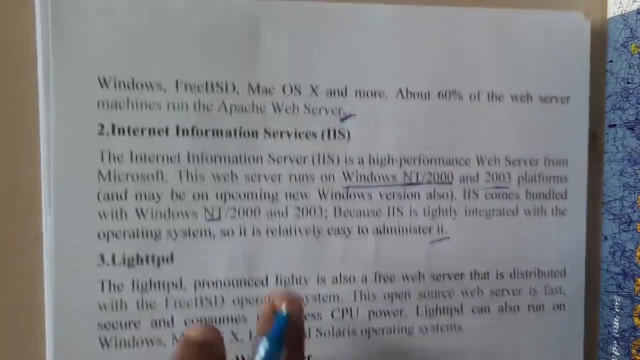 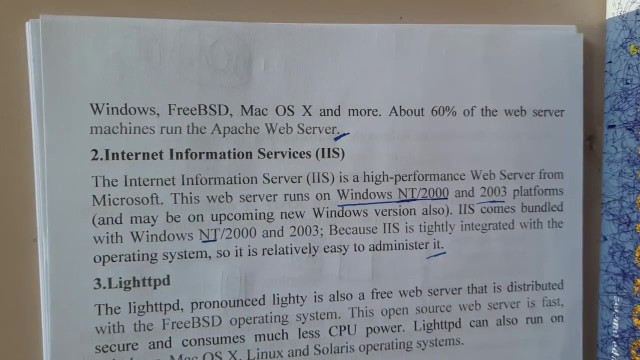 This web server runs only on Windows. Network NT is nothing but Windows Network 2000 and 2003.. Performs and may be, may be on Outcoming new, upcoming new operating systems will also be supported. Okay now, in future, guys? this is not released yet, so it comes a bundled with the Windows NT. that is nothing but Networking 2000 and 2003. so it is inbuilt in those things because these networking operating systems are used for servers only. they'll be using mostly for servers only. so because IIS is tightly integrated with operating system so it is more reliable and easy to manage. so basically, in Apache it will be a bit tougher to come to adjust because it is possible on each and every operating system. so it's a bit confusing. 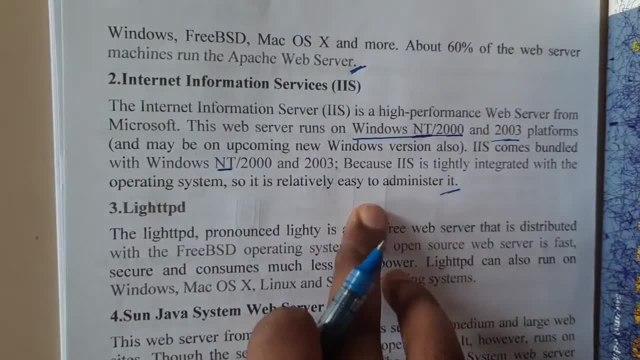 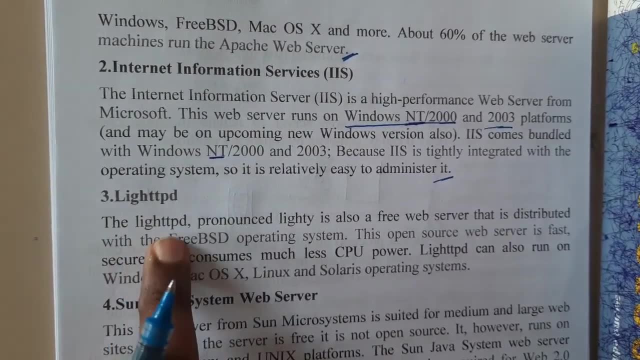 Right, Whereas this is designed for a single process, so it's readability, or understandability, is really high, Okay. Similarly, we are having a Lite TPD that is nothing but Lite TPD, pronounced as Litey, Is also a free web server that is distributed with 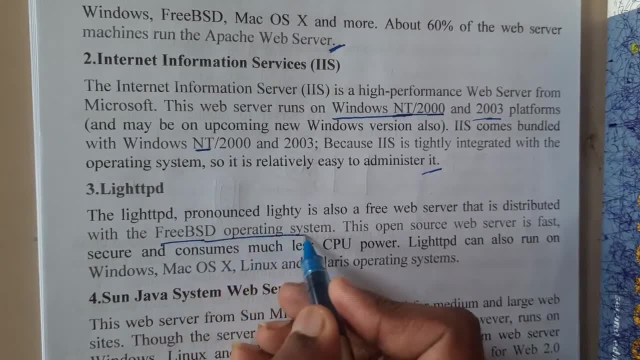 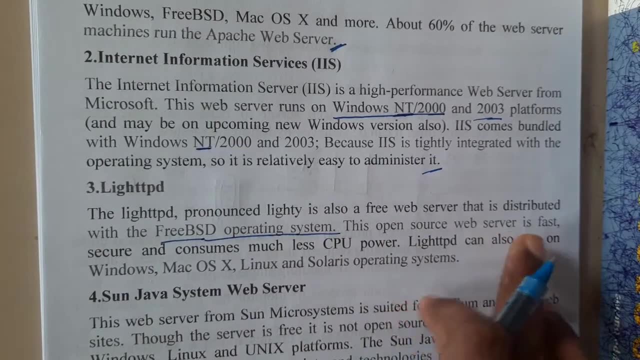 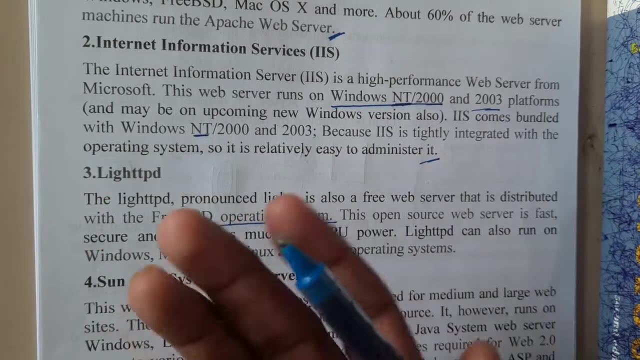 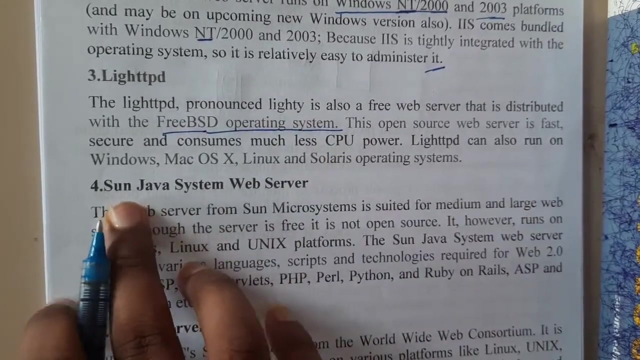 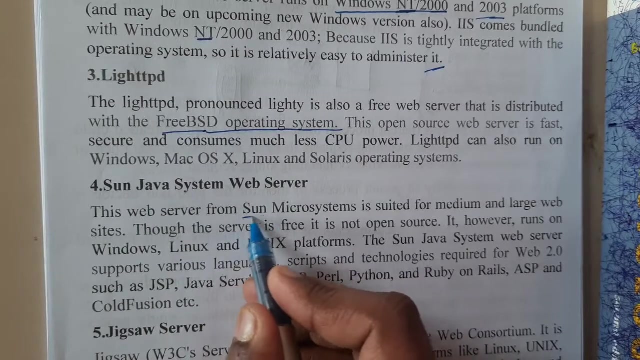 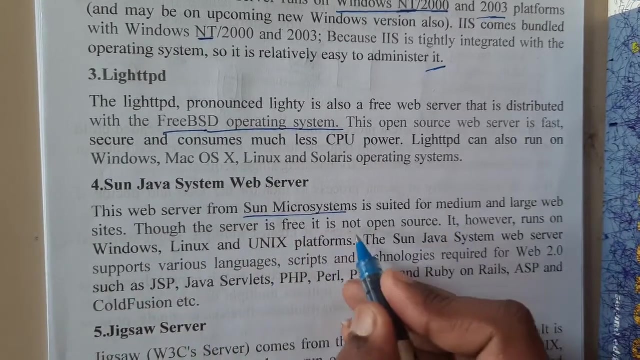 Free BSD. this is an operating system, guys. I was also Seeing this operating system for the first time. I even don't know what is the operating system. so this open- this is also open source, guys, and it is very fast And Consumes a lesser CPU, guys. that is the reason why the name itself is saying that: Litey. it is lightweight CPU process and it can also run on Windows, Mac, Linux and Solaris operating system. okay. similarly, we are having a Sun Java system web server. so even Java also we are having. so this web server is produced by Sun Microsystems. okay, is suitable for medium and large square websites through. though the server is a free, it is not open source. this is the small drawback in this. so it, however, runs.